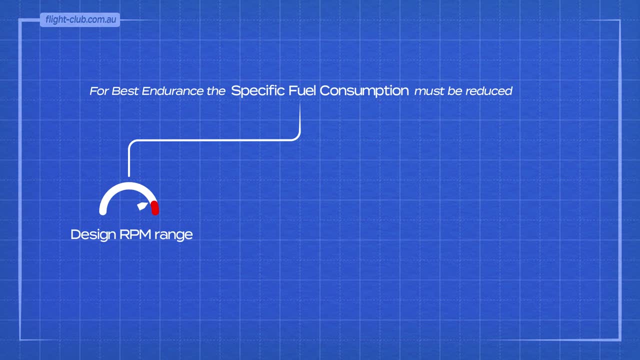 Increased engine RPM does increase the fuel flow, but it also increases thrust. The thrust increases by a greater amount than the fuel flow and this results in an overall decrease in the specific fuel consumption ratio, Which is good for endurance. Specific fuel consumption may also be reduced by flying in lower outside air temperature and higher altitude. 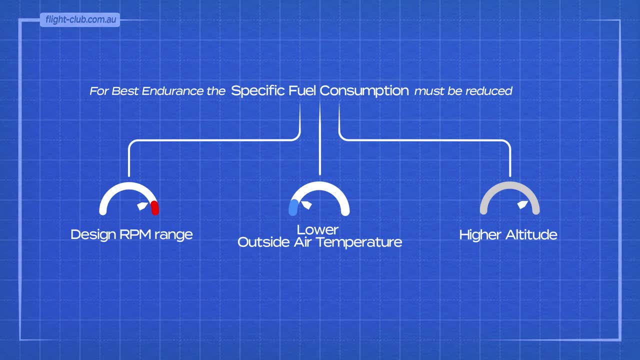 Generally, endurance improves with an increase in altitude, but once the design RPM is exceeded, higher altitude may reduce endurance. Less fuel used for each unit of thrust is only part of the achievement. Less fuel used for each unit of thrust is only part of the achievement. 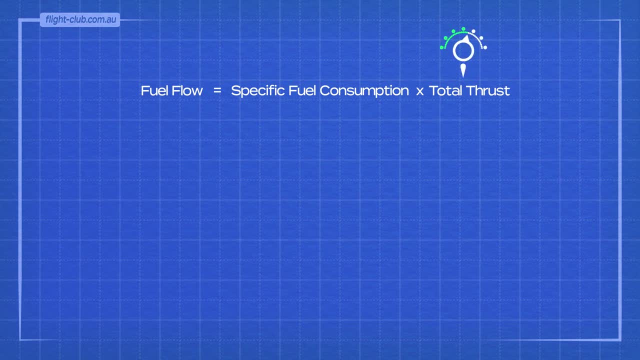 equation. The aim is to reduce the total thrust as well. In level flight, the forward-facing force of thrust is balanced by the rearward facing force of drag. If drag is small, the aeroplane need only fly with a small amount of thrust. In the fuel flow formula, thrust can now be replaced by drag. since the 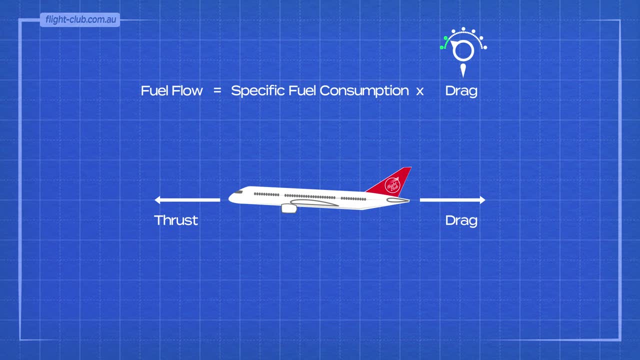 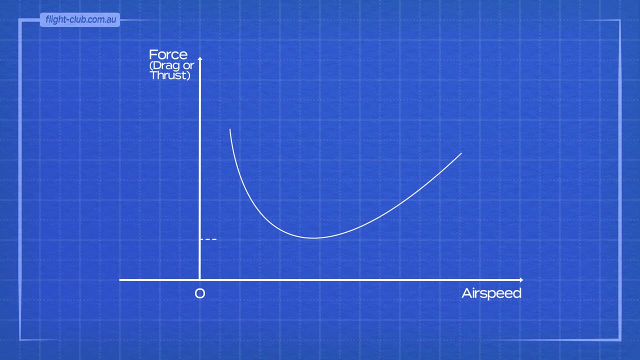 value of drag is equal and opposite to the value of thrust. To minimize drag for best endurance, the jet aeroplane must fly at the minimum drag speed. Minimum drag speed is where the total drag is at a minimum. It is also the speed for best lift to drag ratio and maximum excess thrust. 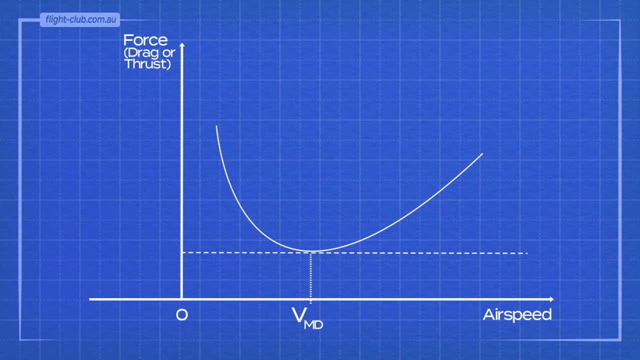 As fuel is burned during the flight, the aeroplane's weight reduces, The drag curve moves down and left. This results in reduced maximum endurance airspeed. The angle of attack for maximum endurance does not change, but the airspeed at which this angle of attack is achieved. 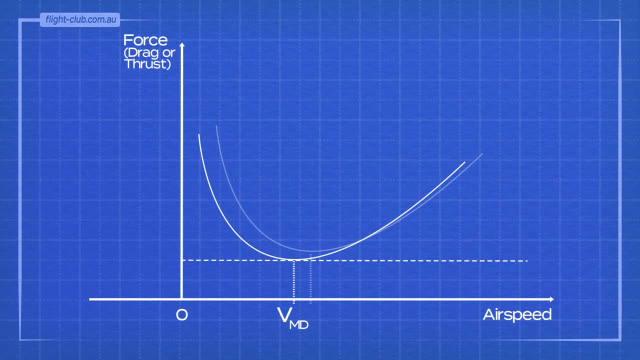 depends on weight and altitude. Subtitles by the Amaraorg community.